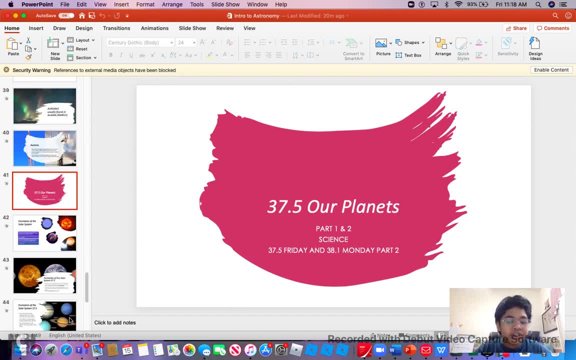 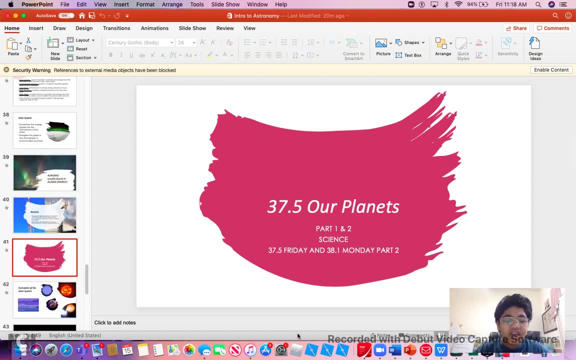 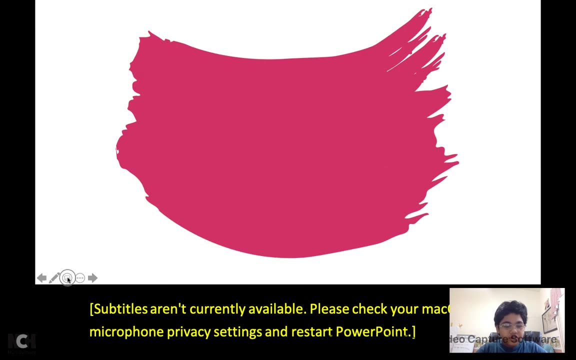 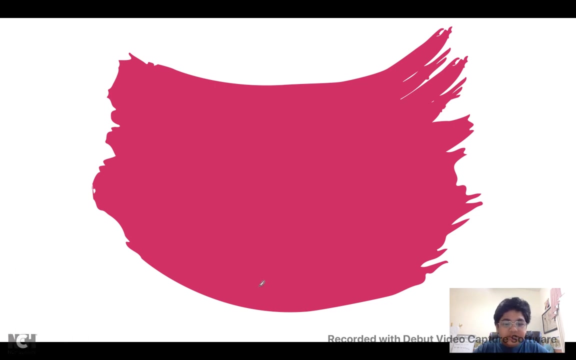 powerpoint. there's only like one, two, three, four, five, six, seven, eight, eight slides, now nine slides. so yeah, but just get started with this video, okay. so today we're going to learn about our planets. 37.5 is today's date, so planets: there's two. 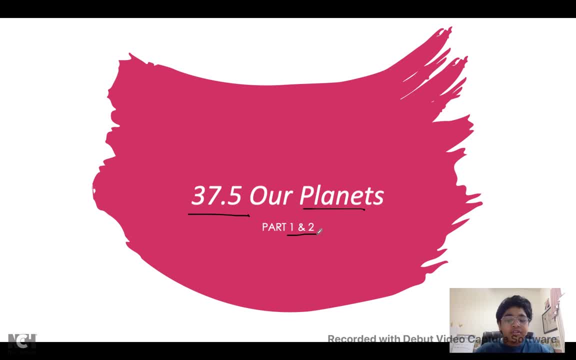 parts this presentation, not this video, though, but this presentation would only cover part one, for today, and Monday would be part two. so, yeah, signs, and so today is 37.5, Friday and 38 point one, Monday. part two would be part two, and today's let's get. 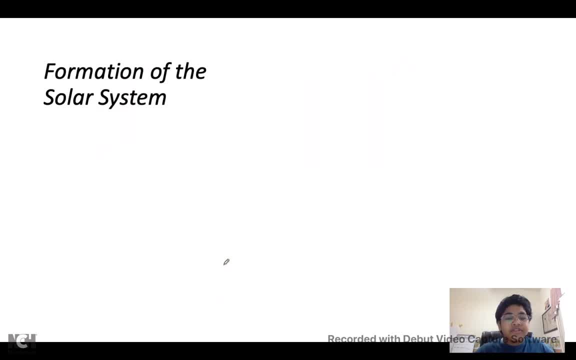 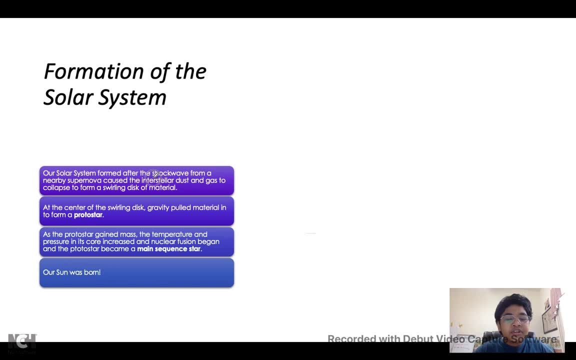 started. okay, so our very first thing. so let's go back to how our solar system was built. our solar system was formed after the shock wave from nearby super mass and low can. part two, and today is day three. today is the third night就 tomorrow. so we're first thing to think a lot about how's it going. 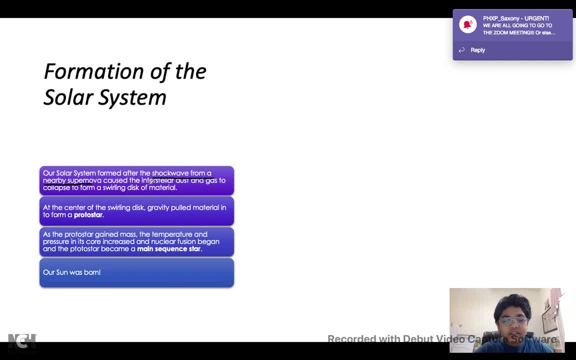 and what the solar system would do on africa. so our solar systems formed after the shock wave zoolittle else over from. It was an actually really hot. oh my god, what a really hot weather was there. Nova caused the interstellar dust and gas to collapse and form a swirling disk of material. 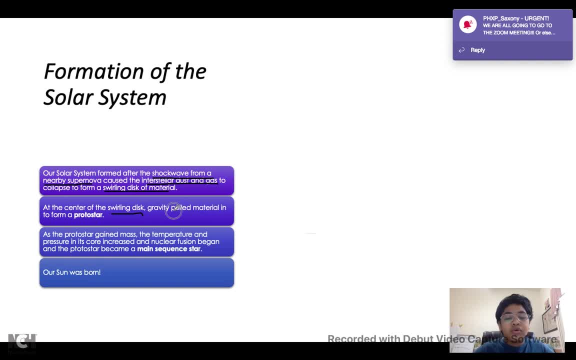 At the center of the swirling disk, gravity pulled material in to form a protostar. If you guys forget what a protostar is, it's a star. right, Okay, just give me Okay. so as a protostar gained mass, the temperature and pressure in its core increased. 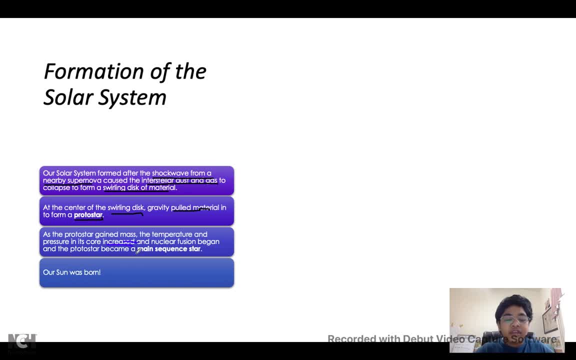 and the nuclear fusion began and the protostar became a main sequenced star And our sun was born. yay, So over here we got a protostar looking nice, Right here you guys can see this is our sun. that was born. 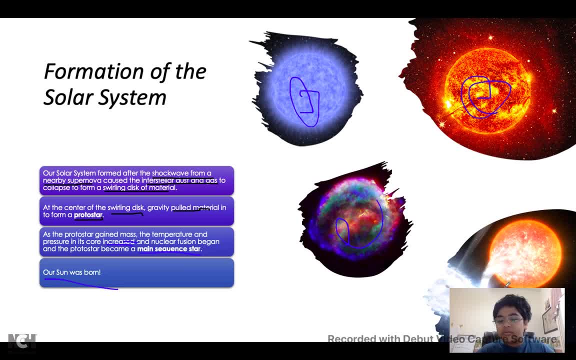 This is the supernova, and no, yeah, And this is. This is your swirling disk. Wait, this is not your sun. This was your main sequenced star. That's your protostar, main sequenced star, supernova. and then that's your swirling disk. 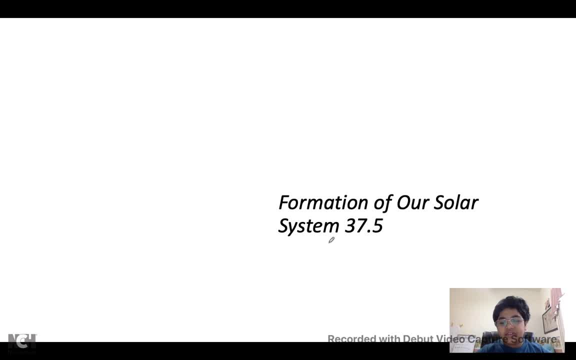 Okay, let's move on. So formation of our solar system continued for today. So, farther out in the swirling disk, material was clumping together and these clumps would collide with each other And pull into other objects to form larger clumps called planetesimals. planetesimals- 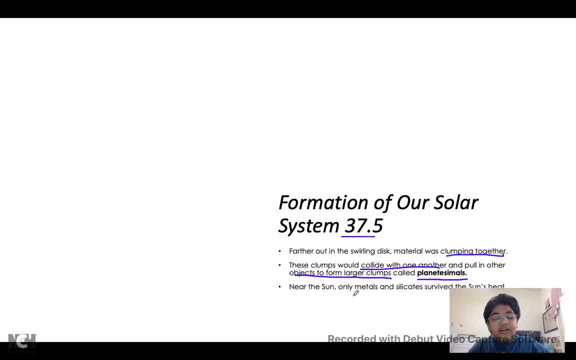 That's a word. that's a weird word to say Okay. so near the sun, only metals and silicates survived the sun's heat. So only metals and silicates were able to survive the sun's heat. As the planetesimals got bigger, their gravity shaped them into spheres. 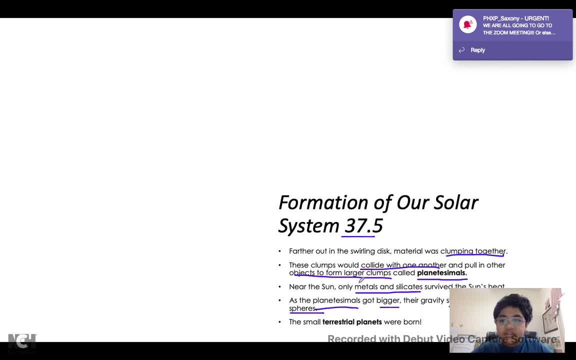 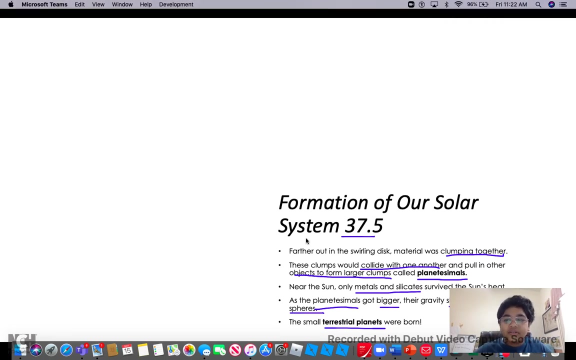 So Whoa? okay, So yeah, the small terrestrial planets were born. Let me just reply to that. Okay, so yeah, Okay so yeah. So over here you guys can see, this is the. 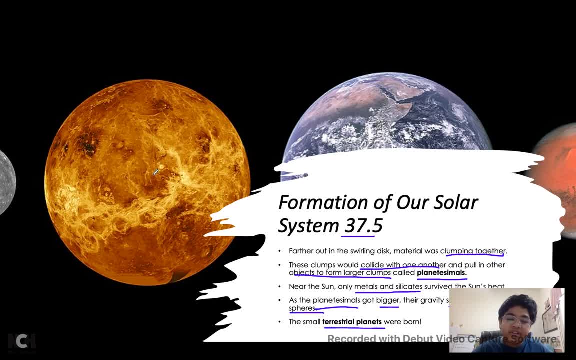 Yes, it's the Yes, it's the Yes, it's the. these are the outer planets or the inner planets that we're learning that today? um, this is your, um, this is the earth, this is the mars. that's mercury right there. you can't. 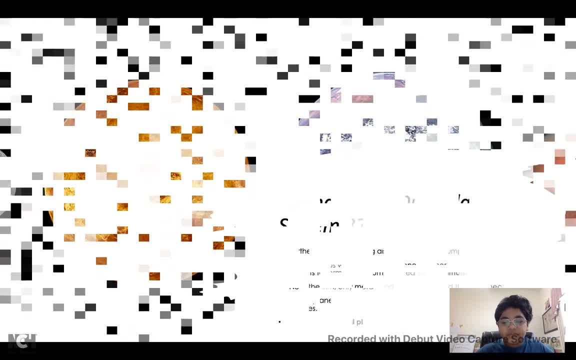 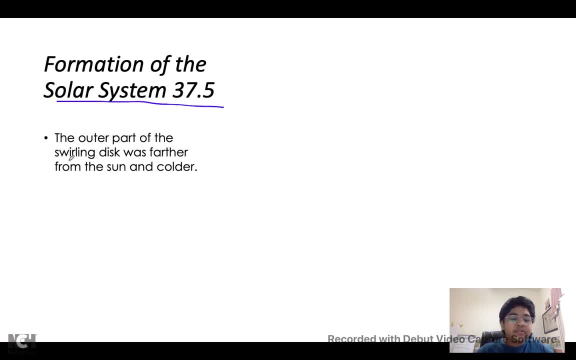 really see it, and that's venus. okay, moving on, so now we can talk about the formation of our solar system and once again so. the outer part of the swirling disk was farther from the sun and colder, and ice, liquid and gas were pulled together by gravity and the outer planets, outer planets, gas. 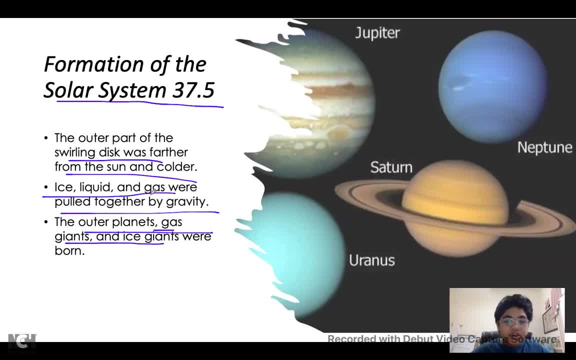 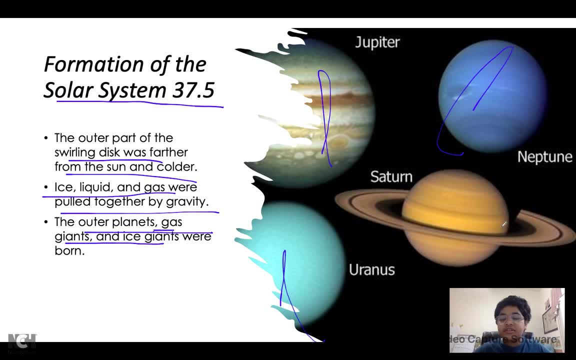 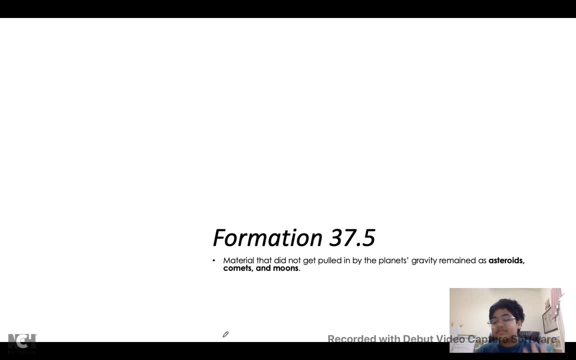 giants and ice giants were born then. so the outer planets, or gas giants or ice giants- jupiter, neptune, uranus and saturn- okay, formation, i didn't want to do formation. some material that didn't did not get pulled into by the planet. planet's gravity remained at asteroids, comets and moons. 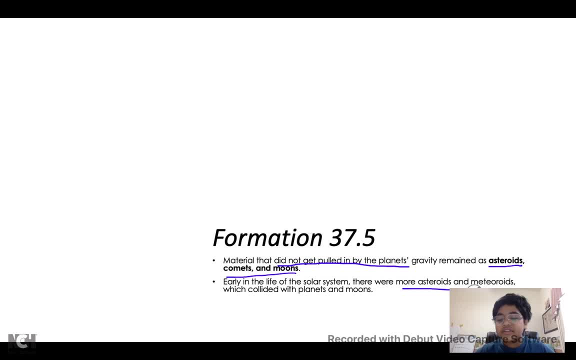 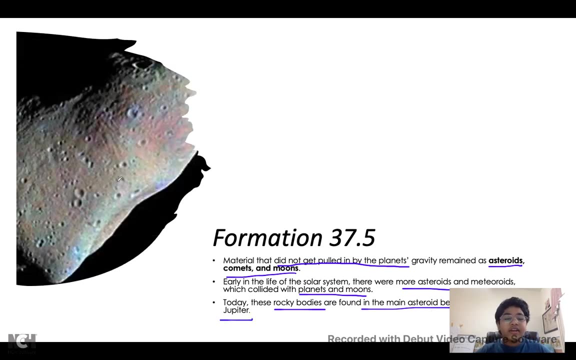 so early in the life of the solar system there were more asteroids and meteors which collided with planets and moons, and today these rocky bodies are found in the main asteroid belt between mars and jupiter. so right here you guys can see this is an asteroid. 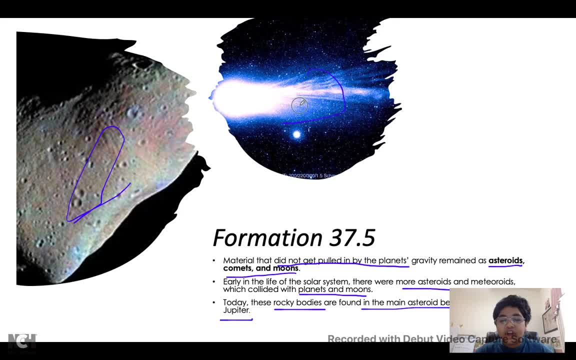 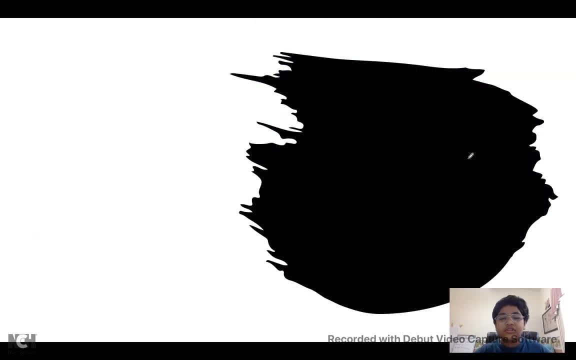 asteroid. over here is a comet and right here is a meteor. i put it in audition, i remember. okay, moving on. so eight planets now. so eight planets orbit the sun in an elliptical order and the planets are the largest objects in the solar system. they're like the largest. 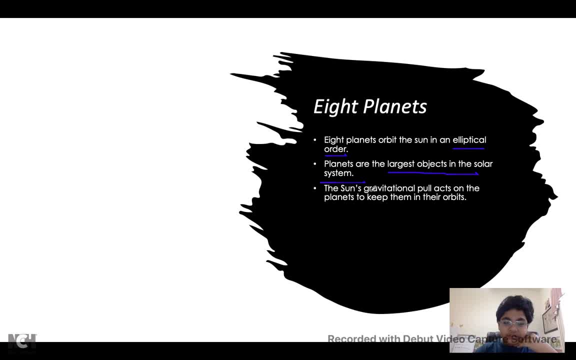 objects in the solar system. i mean the sun should be, but the planets are the largest objects. the sun gravitational pull acts on the planet's, keep them in their orbit. so the sun would do the gravitational pull on the odd planets to keep them in their orbits. mercury. so the a planets are mercury, venus, earth, mars. 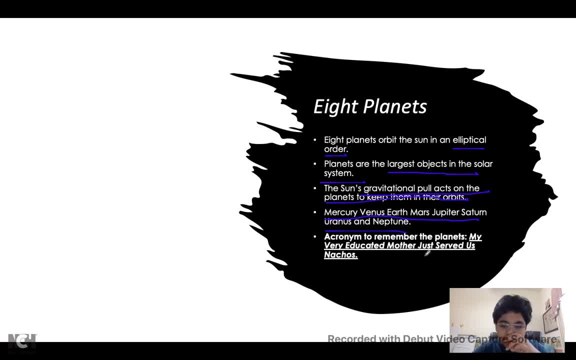 jupiter, saturn, uranus, neptune. and to remember this, you can go my mercury very for venus educated for earth. mother from mars, just for jupiter s were served. you for uranus and n4 septuplets you can go mine very educated mothers just served as, not just 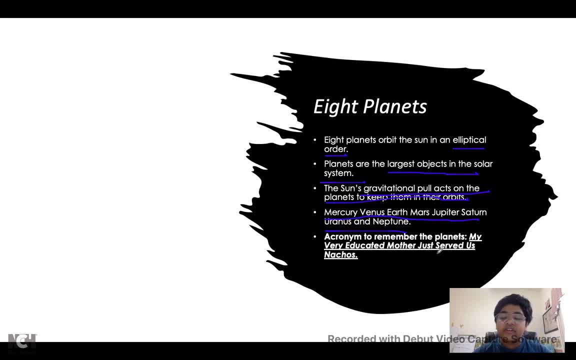 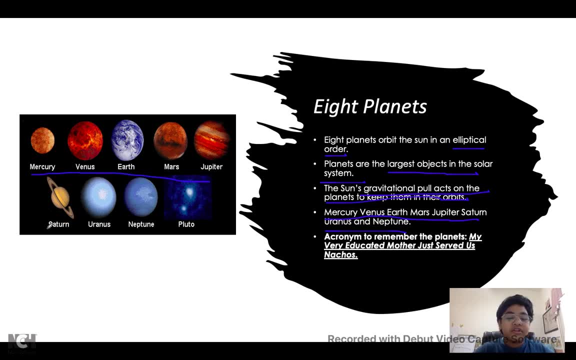 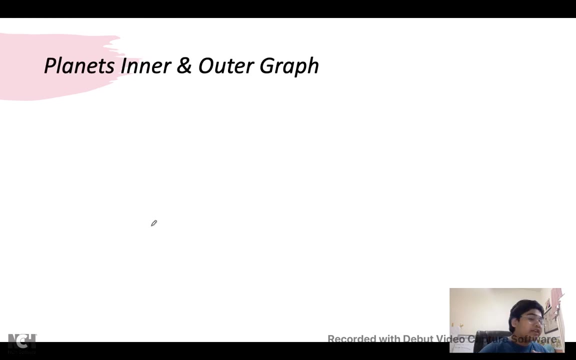 mercury, venus, earth, mars, jupiter, saturn, uranus, neptune. it's cool. so once again, it's in order now: mercury, venus, earth, mass, jupiter, saturn, uranus, neptune. so, oh well, pluto. so my very educated mother just served us not just lacquer up your other acronym acronyms for these eight planets up in here, but i personally like this one. 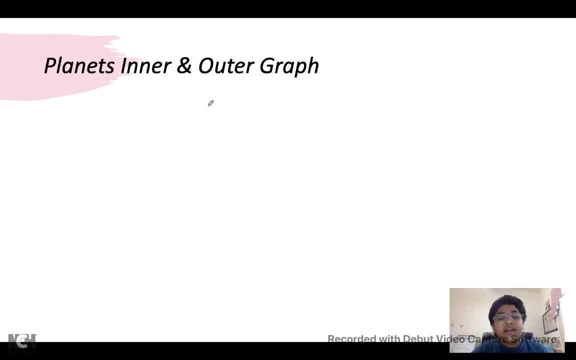 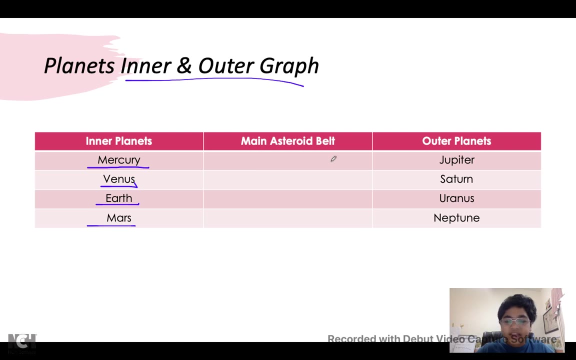 i think that's good, but you can make your own. so planets, inner and outer. so i made this table graph thing. so here it is. so the sun is on your notes as well. so the inner planets are mercury, venus, earth and math, math and mars, and for the main asteroid belt, we're going to learn that on monday. 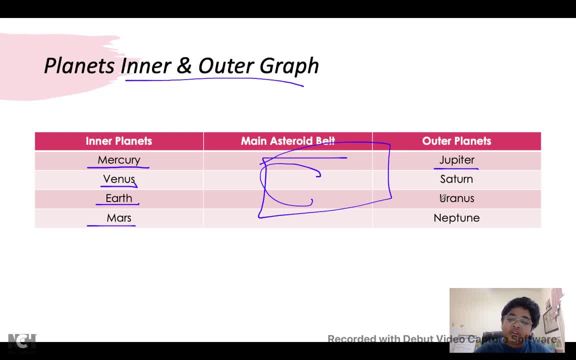 so this will be filmed on monday, i think outer planets is on: jupiter, saturn, uranus, neptune. same thing, mad, my very educated mother just served as nachos. but four of those, the first four that are the closest to the sun, are the inner planets. the one that are photos from the sun are the other ones. 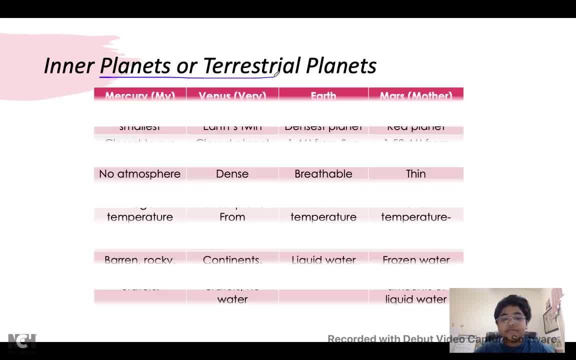 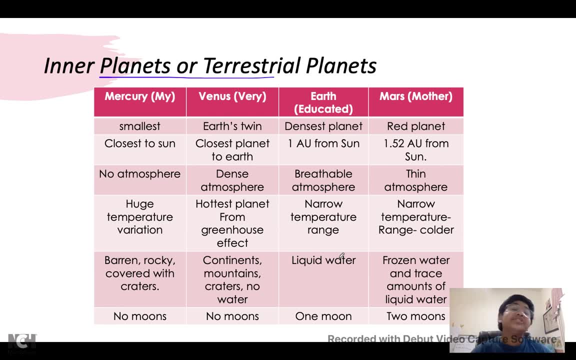 okay, inner planets or terrestrial. so over here in your notes, this has this. my teacher basically made bunch and bunch and bunch of slides. i didn't do it, i just put in this. so the very first thing we're going to talk about is mercury. so mercury is the smallest planet out of these. it is the closest to. 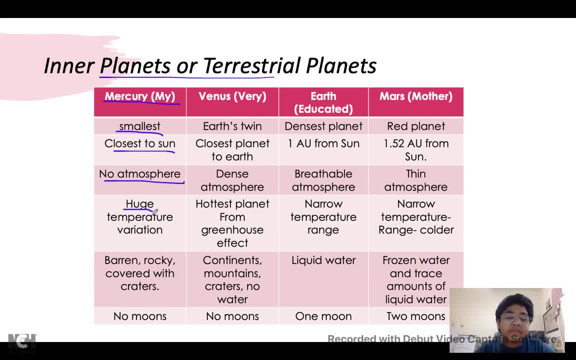 the sun and it has no atmosphere. it has huge temperature variation and it's made of, so its surface is like bare and it's rocky and it's covered with craters and there's no moons on mars. sorry, venus, now venus, so yeah. so i just did the acronyms, so mercury from my. 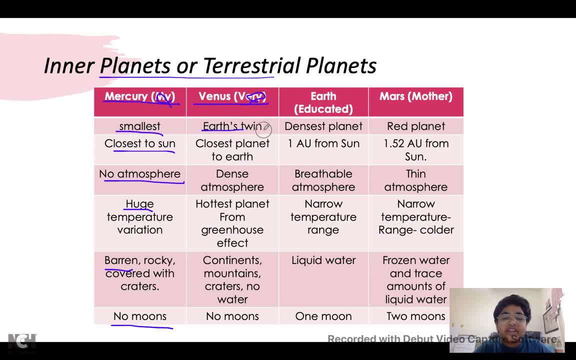 mirror. my venus were buried, so venus is like the earth's twin. it's the closest planet to earth. so venus earth, they're close together and it's it has a dense atmosphere. it's hottest planet from the greenhouse effect, so the greenhouse perfect. probably happened here. 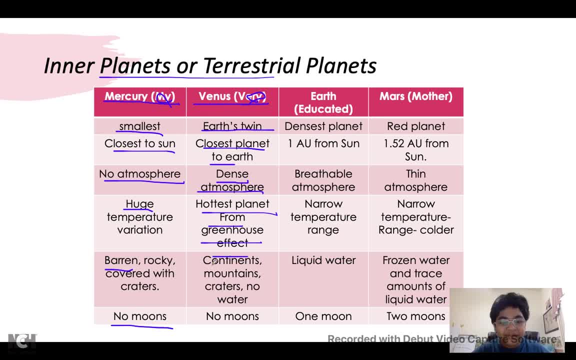 and then it made it the hottest planet on the earth. so so i forgot to add this. but on the world, or on its globe, they did this colorful thing where they would continent this area, mountains, this area, cretus, radars that area, and if there's no water, they did it, that area. 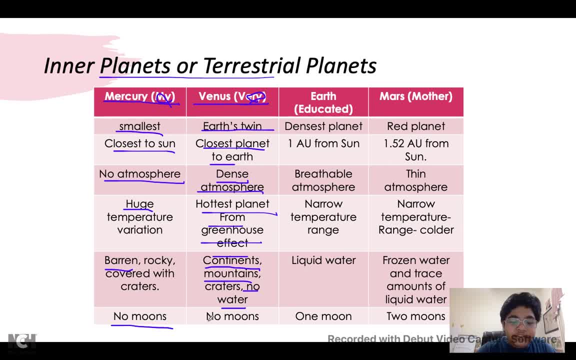 i didn't put it in here, but you don't need to know that, actually. and also, venus also has no moons. sorry earth. yeah, it's our earth. it's educated- yeah, we are educated. okay, so densest planet, this is the, this planet of all. so it's one astronomical unit from the sun. it has a breathable atmosphere, that's. 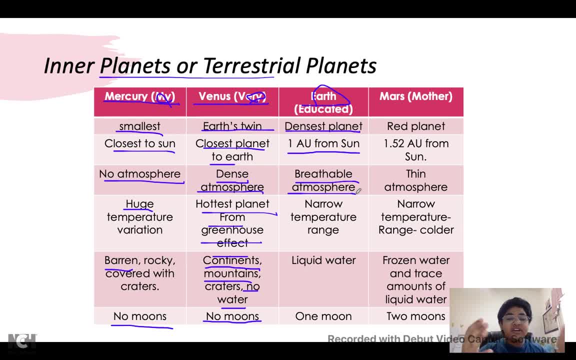 why around me i can breathe. so i can tell you guys the information you know: breathe. it has a narrow temperature range. i mean, like in the summer it's so hot in phoenix, arizona and everywhere maybe. and yeah, it's able, it's capable of having liquid water and it does have one moon, you see. 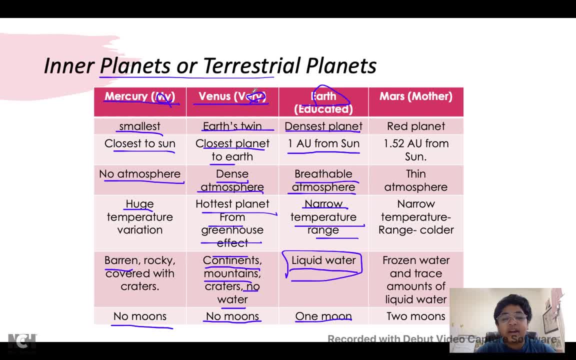 that night time. so, yeah, this is educated and i'm very educated. and then the last one, mother for this week, on friday mars. so it's a red planet. it's like covering is kind of red. so basically, the dust storms kind of- yeah, the dust storms got color and they colored it all red. 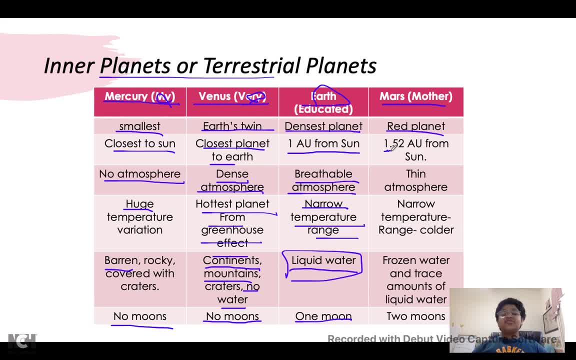 i think, yeah, so that's what my teacher says. she's like, okay, so it's red because of all the um, because of all the storms that happen, which change the color of their atmosphere, change the color of the soil. so yeah, and there's one point about 1.5 to 1.5 astronomical units from the sun, and it has a thin. 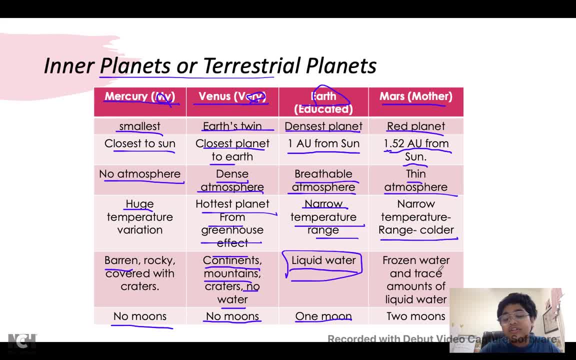 atmosphere and its narrow temperature range is colder and so, yeah, mars is colder. so usually at night time it goes up, down and during the day it's also kind of down. but you know medium and mars, frozen water and trace amounts of liquid water, so frozen water. so they're still looking for frozen water, but there's. 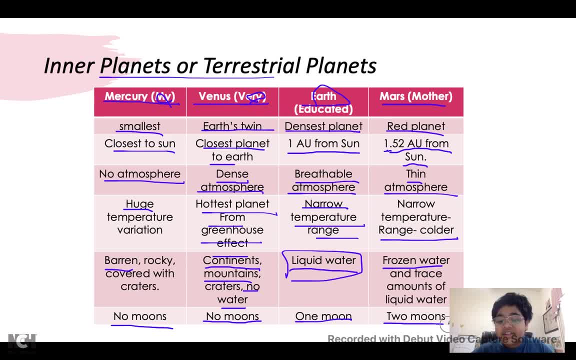 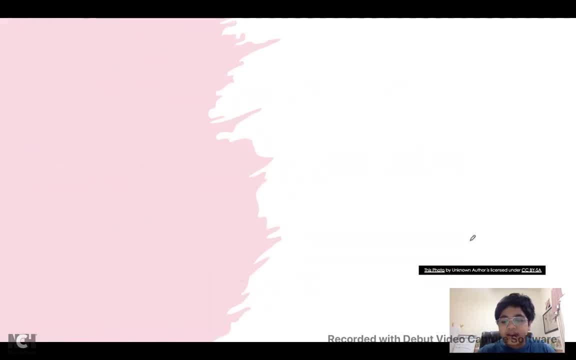 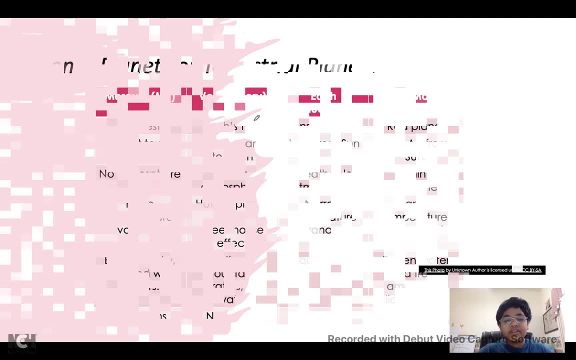 some trace amounts of liquid water in there. and mars is lucky, he has two moons, so you see two moons at night time. cool, okay, uh, last slide. yeah, so inner planet or terrestrial planet? i you know how I did this to this. I put it here. but what's gonna happen is there was two. 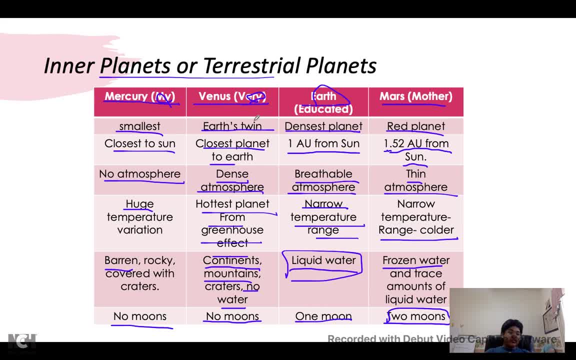 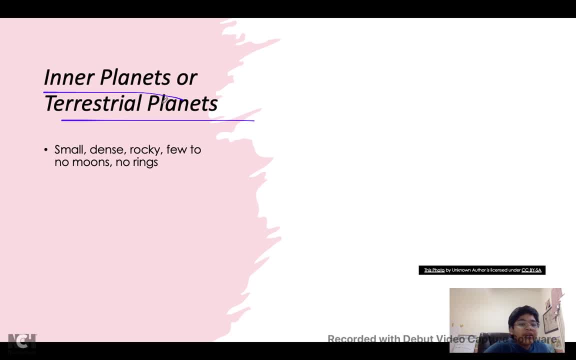 lines before this graph. I didn't put it in here- there's no space to, so I bought it here and put it in here. so so inner planets, basically, or terrestrial planets. so they- they're either inner planets or terrestrial planets- are small, they're dense, they're rocky and they're few to no moons and then no wings. and these